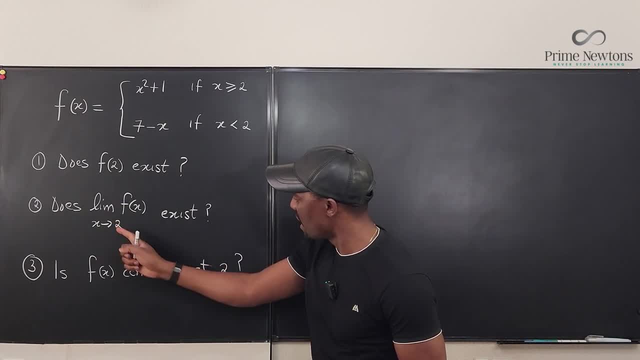 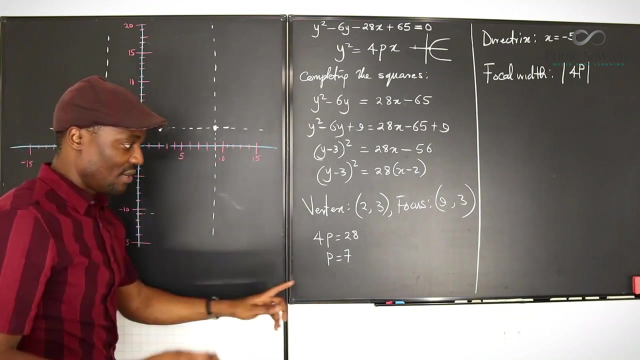 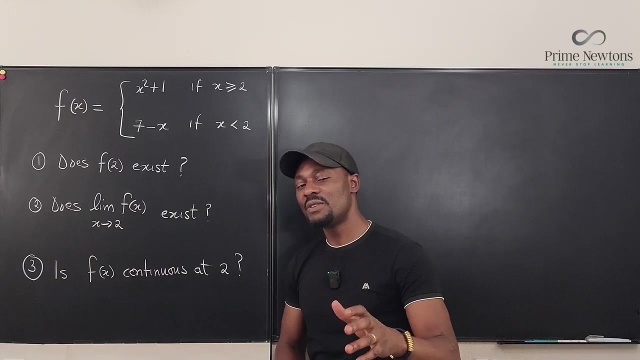 focus of everything, and every question you've been given has focused around 2.. So that's the point. The question is: is it continuous at 2?? Let's get into the video. So here is the answer to all of these questions that you see on the board and the ones you have on your mind and the ones I have hypothesized. 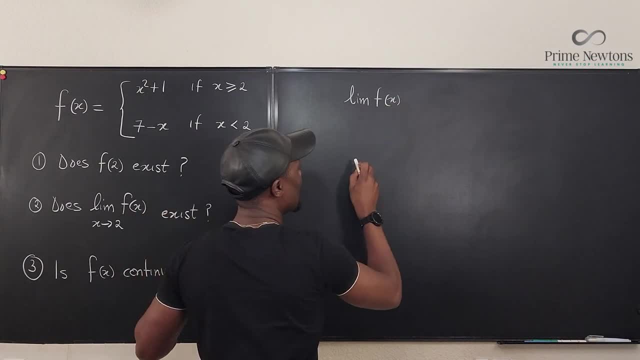 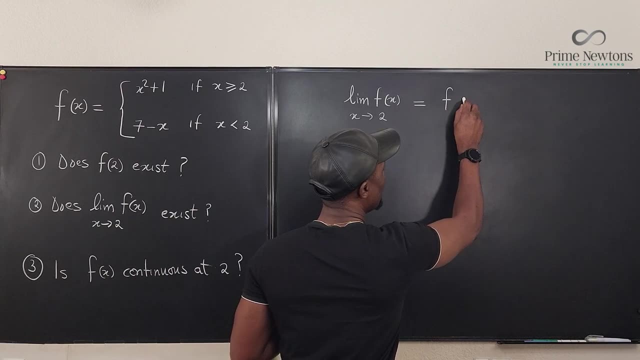 The limit of this function, as x approaches 2, is equal to the value of the function at 2.. This is the answer to every single question that is here. There are three things that must happen for a function to be continuous at a point. 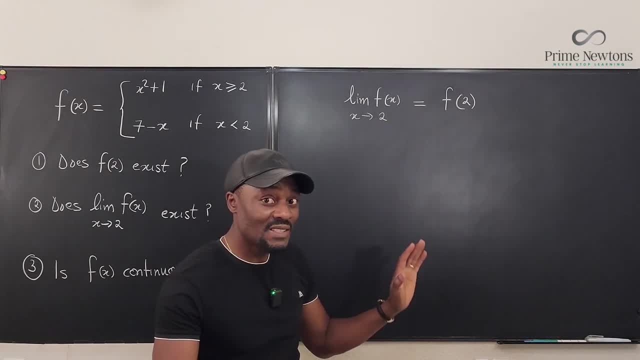 In this case, it's a two. See, there are three things that must happen, and the three things are written on the board. The first thing that must happen is this: This has to exist. See, when you have an equation. 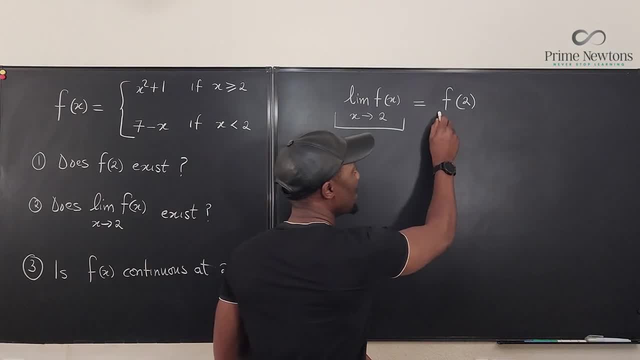 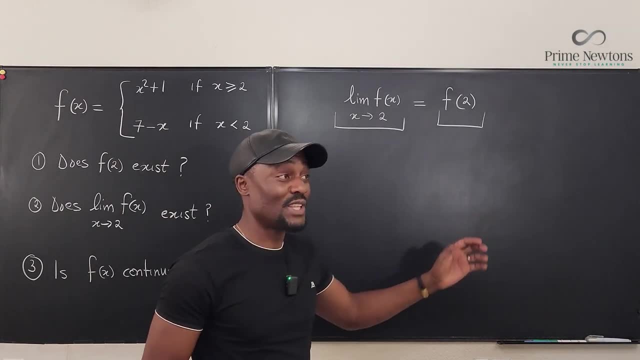 the left-hand side and the right-hand side must exist for the equation to make any sense, and this is the continuity equation. okay, Just as you have Einstein's relativity equation, or whatever. E equals MC squared. Yes, this is your: E equals MC squared. 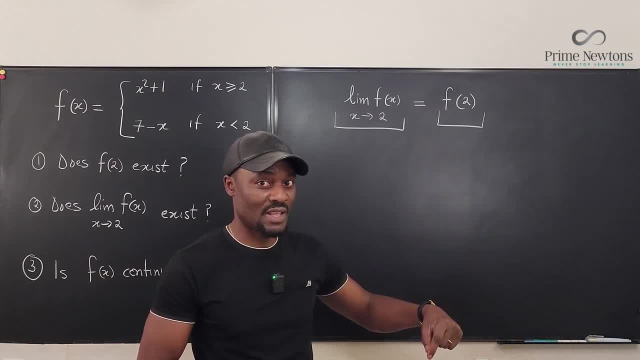 for continuity of a function at a given point. So this must exist and this must exist. What is the third thing that must exist? This must exist, All three must exist. If one does not exist, then the function is not continuous at that point. 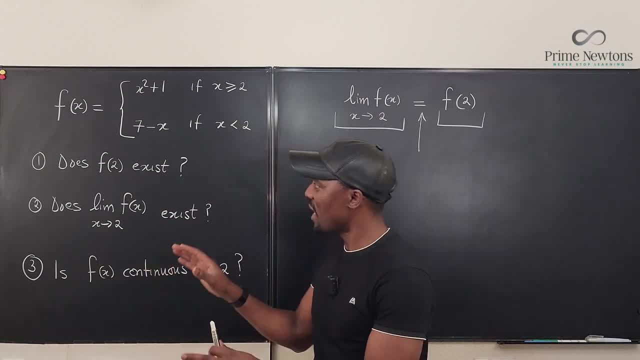 So, with that understanding, we're gonna go back and try to answer each of these questions and then we'll come to answer this final one, whether f of x is continuous at two, because if we don't get that, it's not continuous. 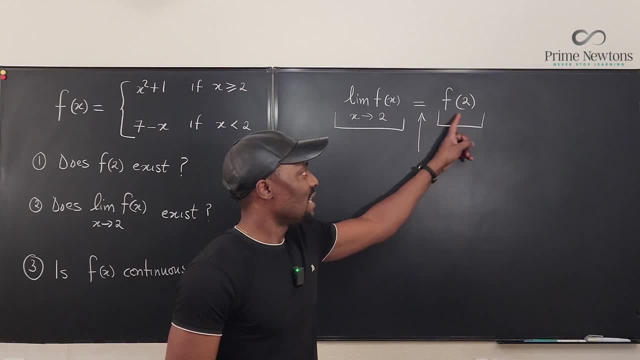 So let's go. Let's start from the right-hand side. What is f of two? Remember that the value of a function at a point is basically what the y component is gonna be. So you plug in two into the function. What do you get? 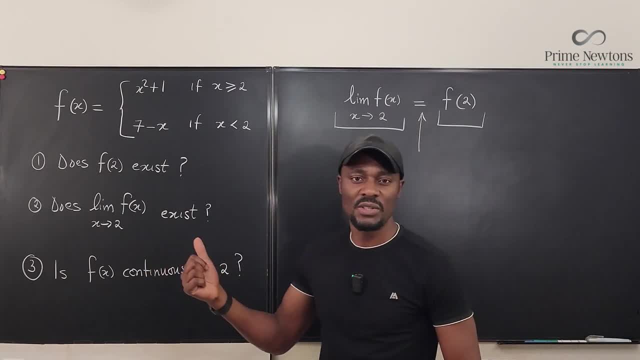 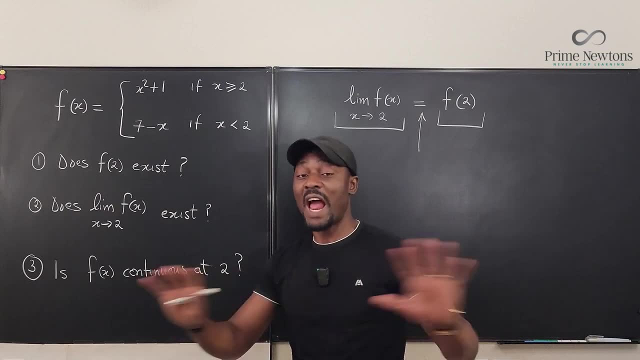 That's what you get here, So do you think we can plug in two into this function? Let's go back here. The function is a piecewise function. I was thinking of sketching graphs to show you how it works, but I don't wanna use a graph. 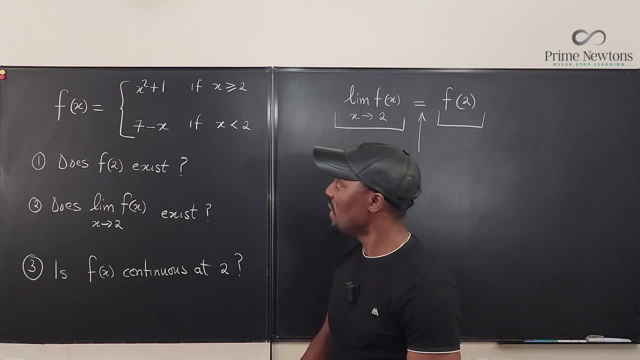 so that your understanding will be based on what you see. So look at this. This function is defined in two ways, depending on where you are on the graph. okay, So any time x is greater than or equal to two, this is what the function behaves like. 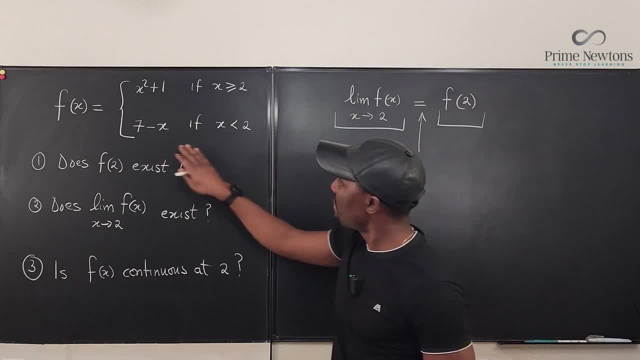 But whenever x is less than two, the function behaves this way, So it's a piecewise function. It's definitely broken. It's a broken function. okay, It has two different parts that don't look alike. But when I want to find the value of f of x, 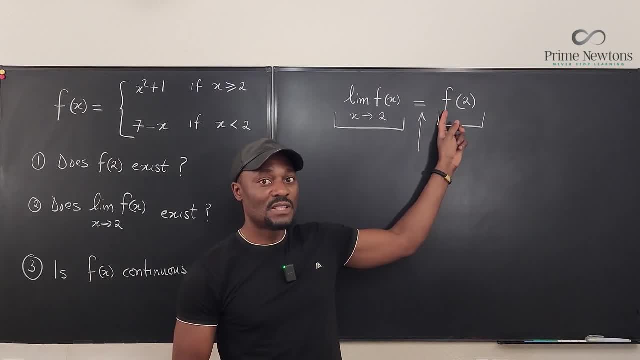 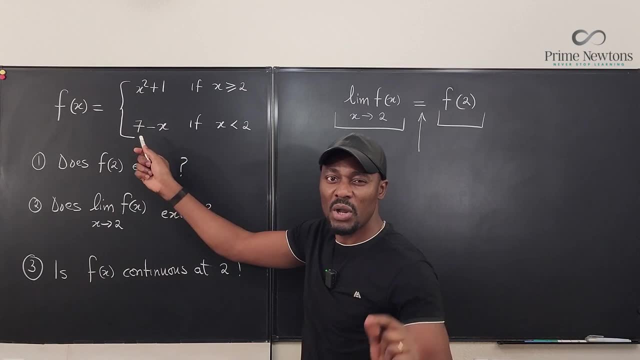 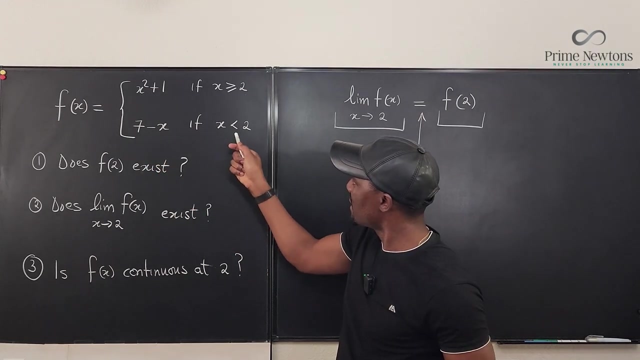 at two the value of this function when x is equal to two. am I supposed to go here to find it? or here? Where should I plug my two into You? plug it when x equals two. Well, x is not equal to here because x is less than two. 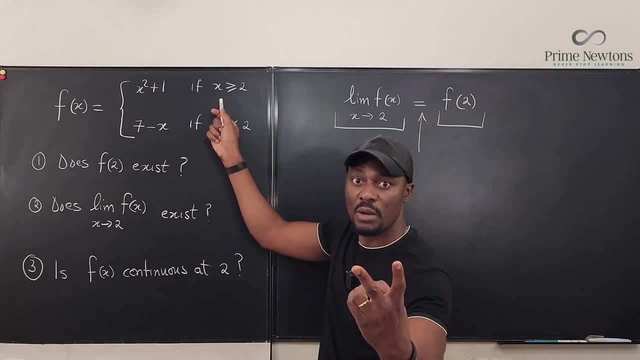 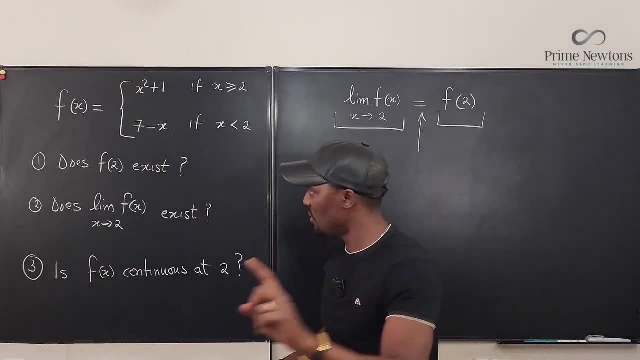 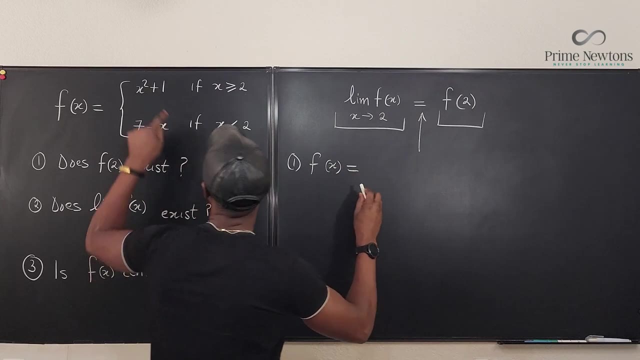 But if you go here, x is equal to two, because you have two options: X is either greater than two or equal to two. So this is the function you're gonna use. So the first question that we're gonna answer is: one F of x is equal to this function. 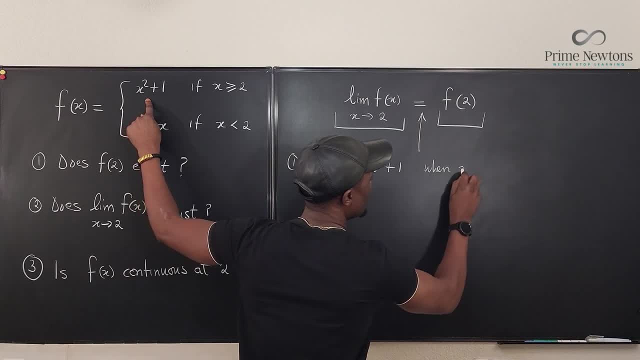 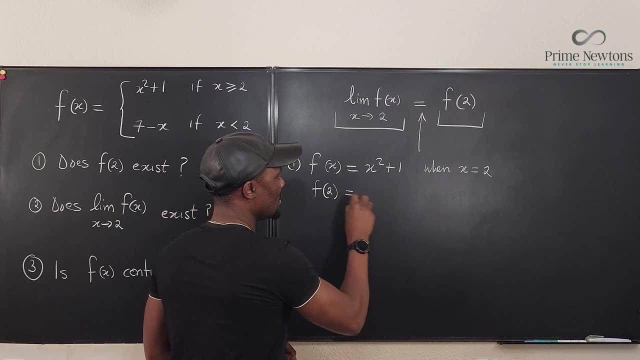 x squared plus one, when x is equal to two. So that's the part you're gonna take, And then you plug it in, So you say: f of two is equal to two squared plus one, which is equal to five. So yes, the first answer has been provided. 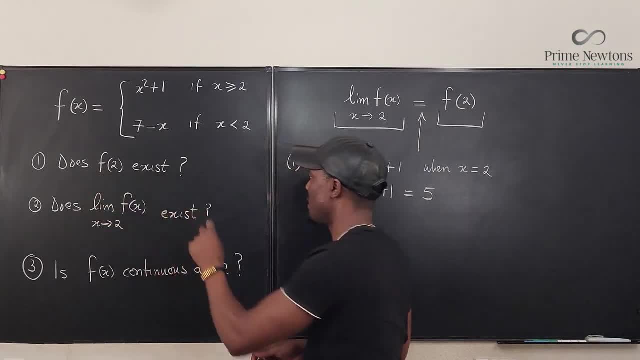 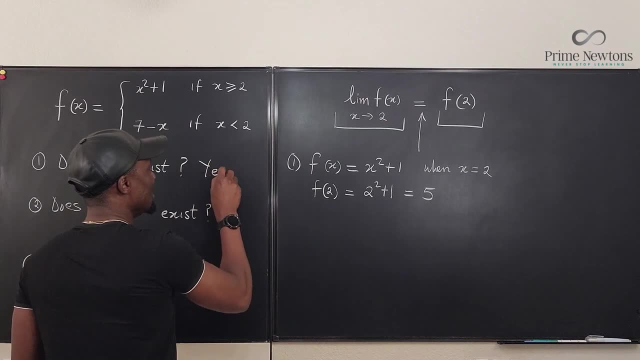 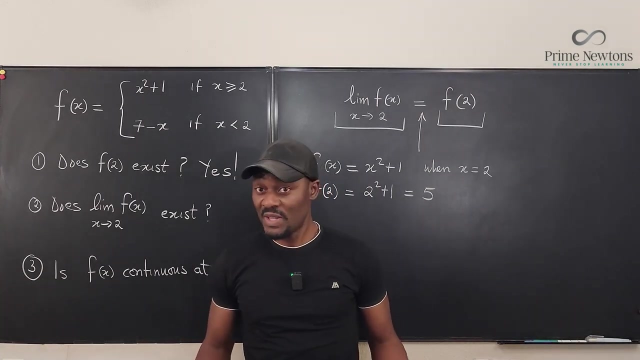 to this first question question: does f of two exist? the question is: does five exist? yes, five exists. so we say yes, yes Lord, yes, Lord. and then we move on to the next one. so the next question says: does the limit of the function as X approaches to exist? 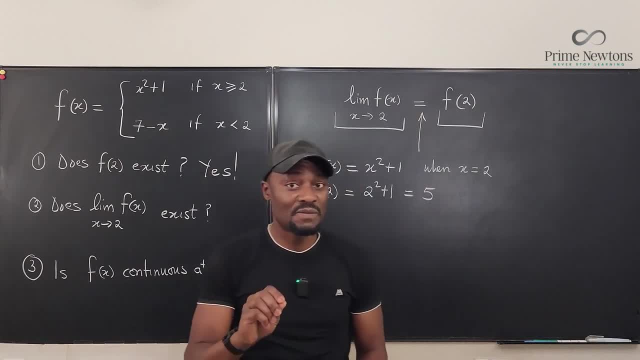 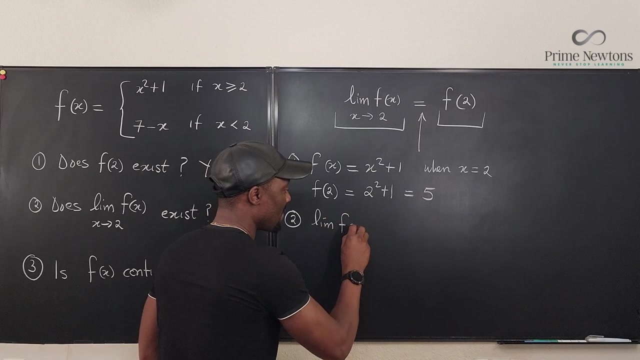 now that's another question. the limit of a function only exists if, as you approach that point from the right, it is the same thing you're gonna get as if you approach it from the left. so remember, the point of interest is 2. so let's go to the second question, 2: what is the limit of this function? as you, 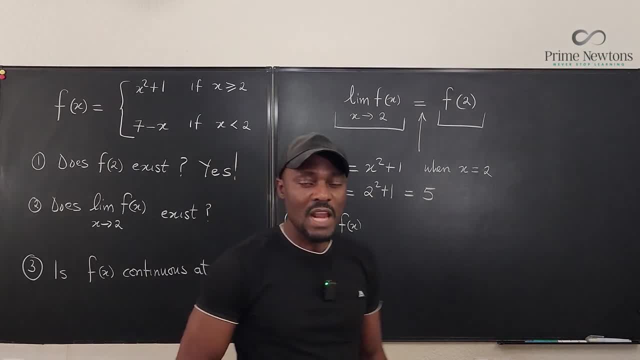 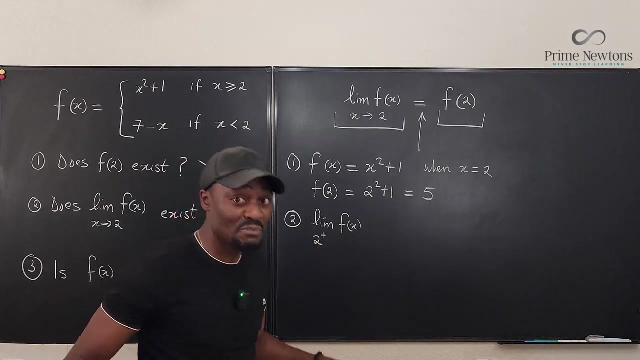 approach 2 from the right. now, when you say from the right when it comes to taking limits or generally, you're saying you're using values that are slightly great than the point where you're talking about. so approaching from the right does not mean positive. so this plus does not mean positive. it means I'm approaching. 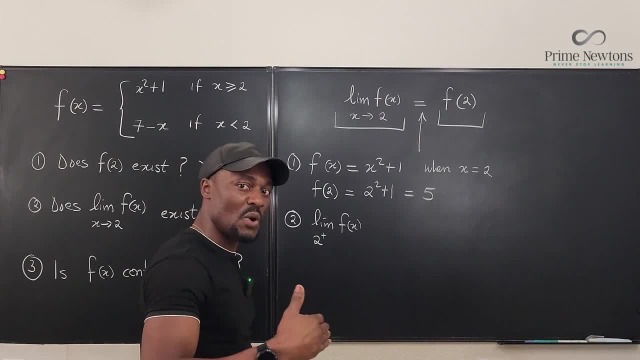 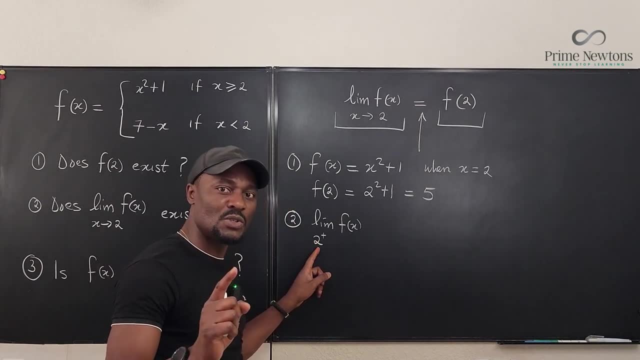 2 from numbers greater than 2. ok, if I'm approaching. however, if it's, if plugging into is not a problem, just plug it in. but wait, what is the function you're supposed to use whenever the value you want to plug in is greater than 2, or you? 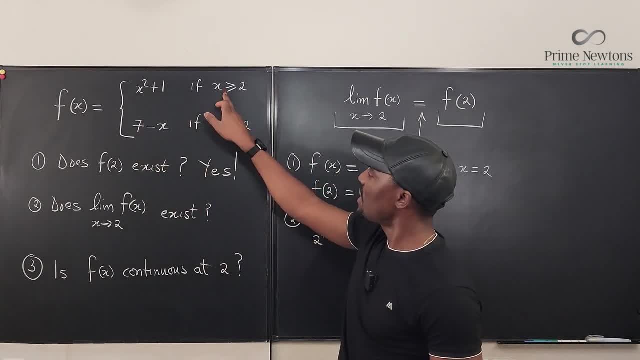 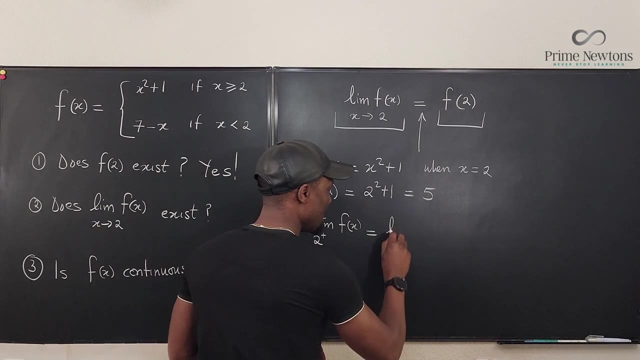 using this function or this function, see this says this is good for values of X that are greater than 2.. So you go back again and say, in order to find this limit, I'm going to plug it in to this function. So it is the same thing as the limit as x approaches. 2 of this is: 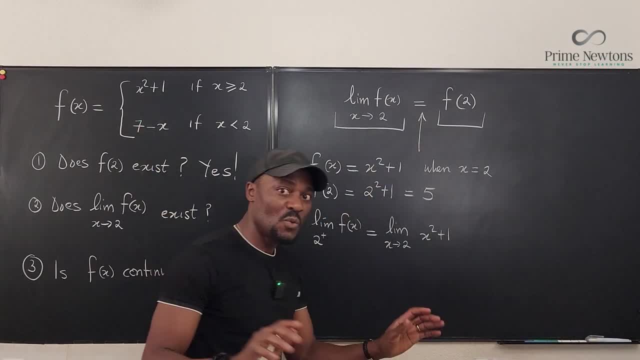 the function x squared plus 1.. And remember, when you take limits- and this point is a finite point, not infinity- your first move is to plug the 2 in right. That's how you find limits. So plug 2 into. 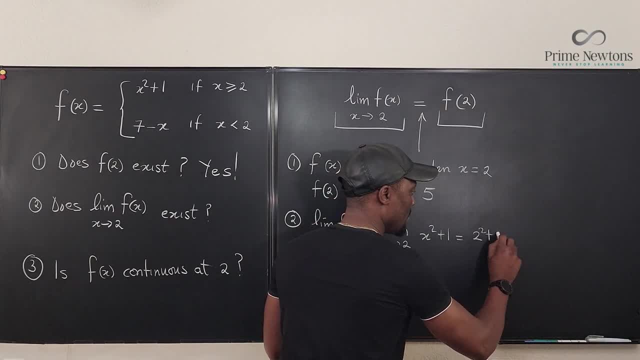 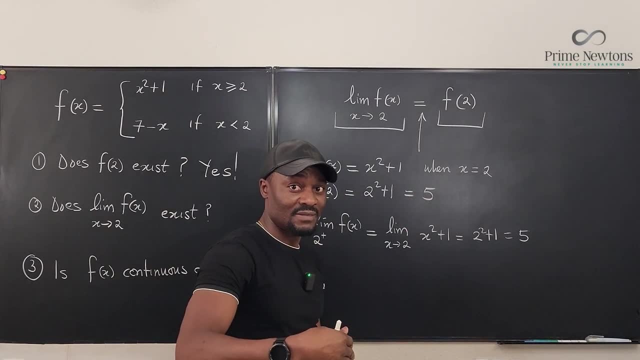 this function. what do you get? You're going to get 2 squared plus 1, which is equal to 5.. You've got the limit as x approaches 2 from the right. So what do you do next? You go back again and say: 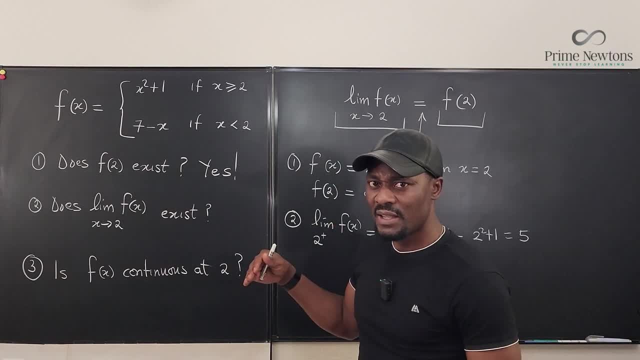 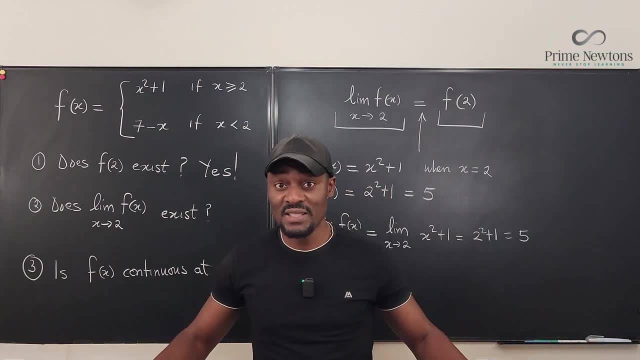 okay, now I know what's going on. if I'm approaching from the right, I'm going to get 5.. What if I approach from the left? Because if the two of them are not the same, the limit does not exist. If the 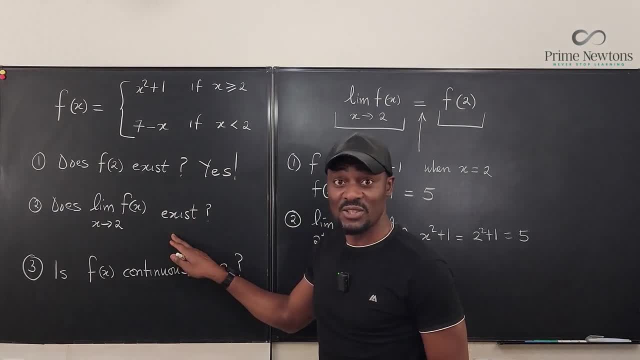 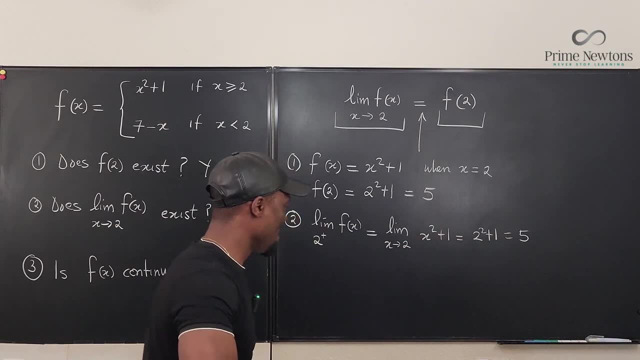 two of them are the same. the limit exists, and that's when you get the answer to this. So this is the limit. This is not the answer. This is just a part of the answer. So let's go. We're going to say now: 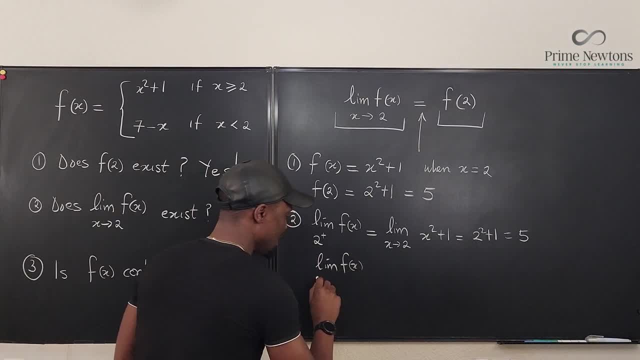 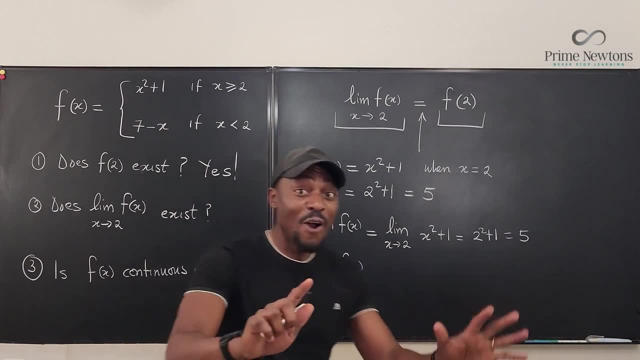 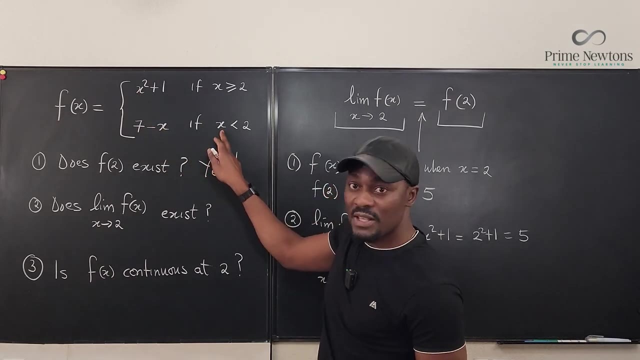 what about the limit of this function as x approaches 2 from the left? So we're now coming from the left-hand side, We're using numbers less than 2.. Now go back to the function. You can no longer use this to compute your limit. You have to use because this is what you must use when 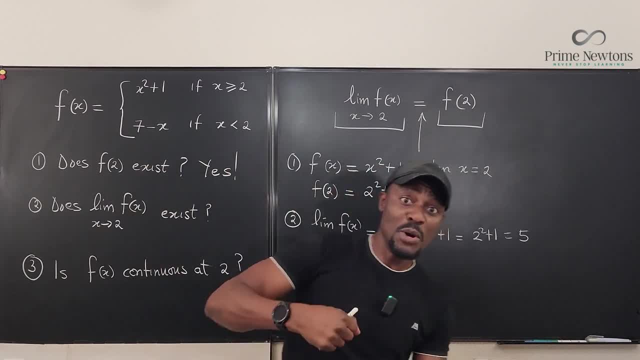 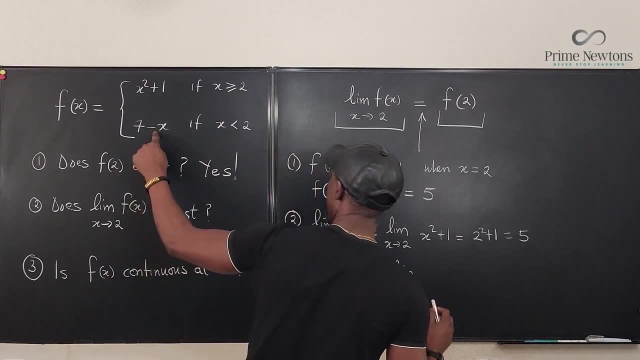 the numbers are less than 2.. So you go here and you plug it in. Boom, Let's go. This is going to be equal to the limit as x approaches 2 from the left. And from the left. this is the function we use: 7 minus x. Well, that's going to be 7 minus 2, which gives us 5.. 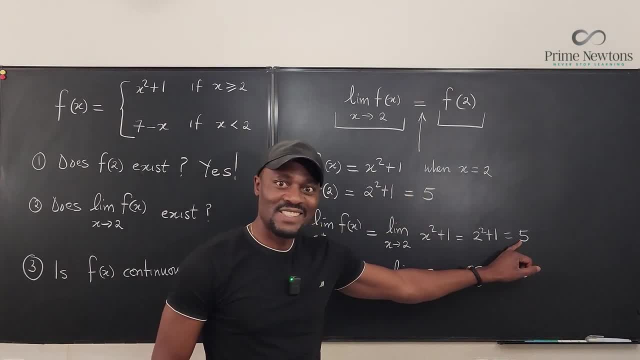 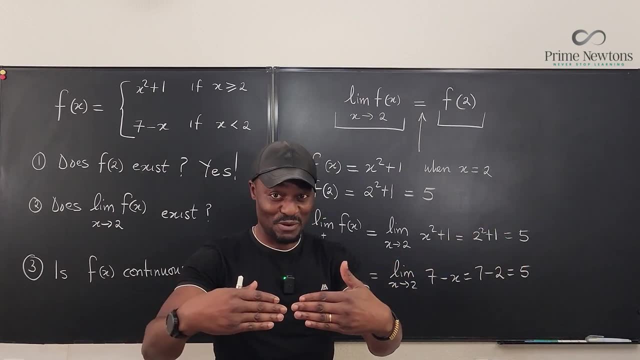 Oh my, This and this are the same. So the limit as you come from the right is the same limit as you approach from the left, And if both of them are the same, then the limit exists, and that is the limit. 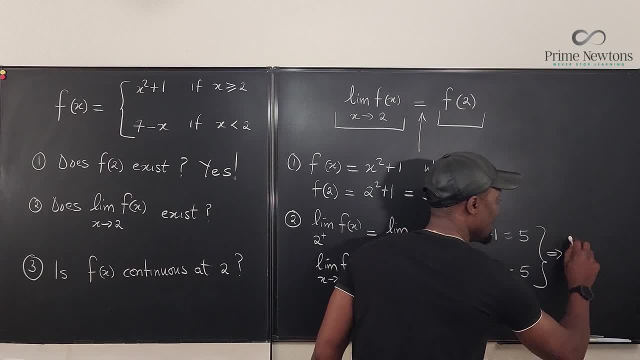 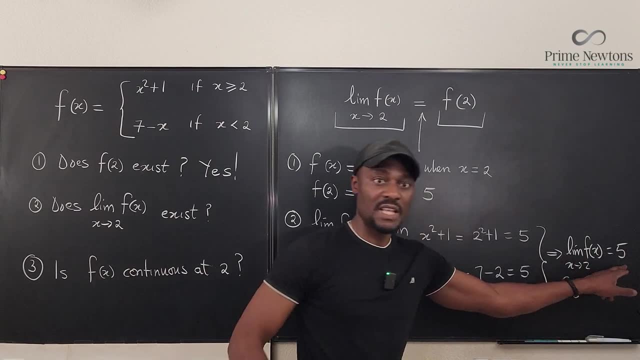 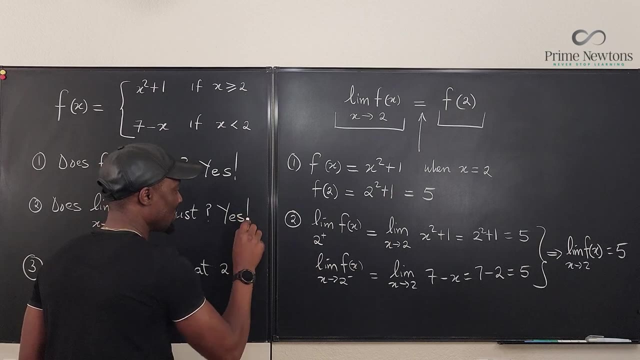 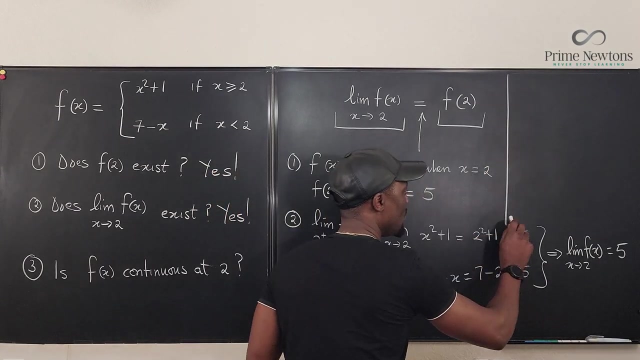 By means of this. this implies that the limit of f of x, as x approaches 2, is equal to 5.. So it exists. The answer to the second question has been provided. Let's go. The answer is yes. Well, we've shown the work. And the final question. I'm going to answer it here. You tell me, Remember. 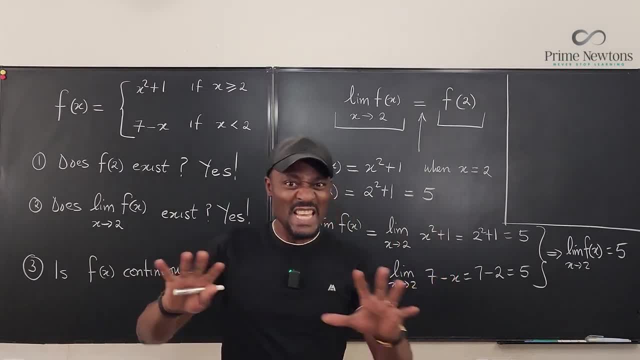 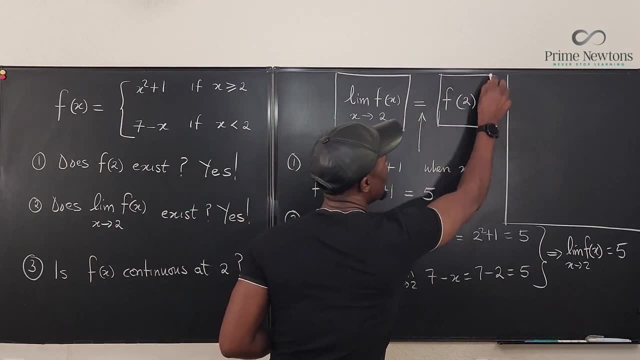 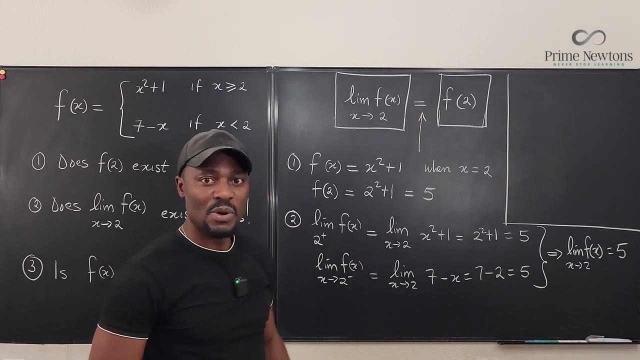 what I told you: The continuity equation. The continuity equation is what I wrote here. This is it. It is the king of everything you are doing. This exists. We started with this. This exists, And this is the middle part. Do you think? 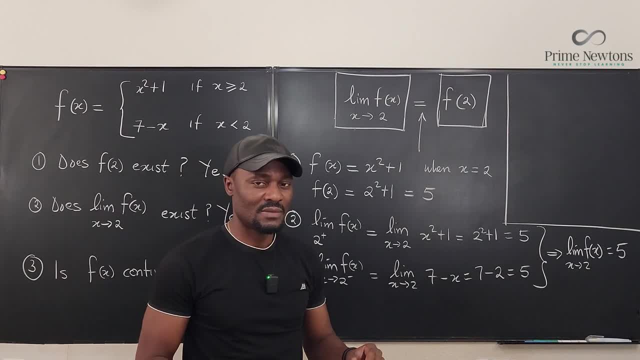 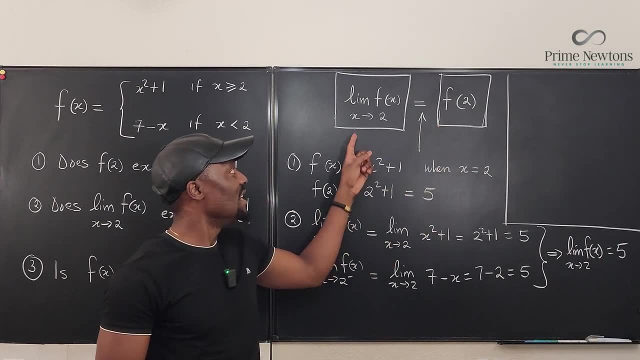 the equal sign exists for this equation. It does Why? Because f of 2 is 5.. The limit as x approaches 2 is also 5.. So this guy is right. So the limit as x approaches 2 is also 5.. So this guy is right. 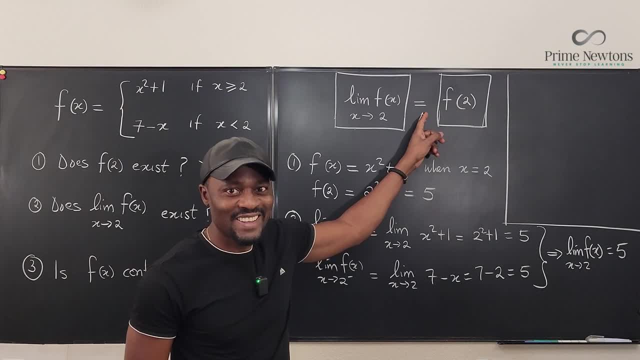 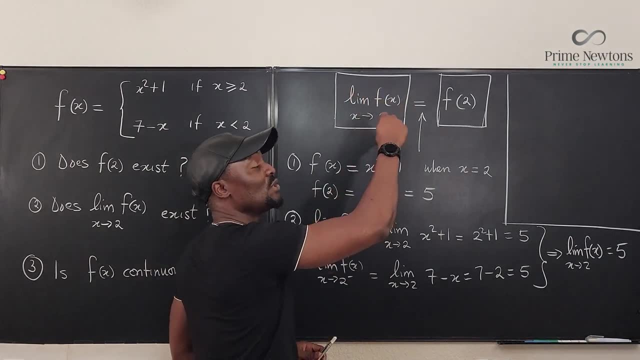 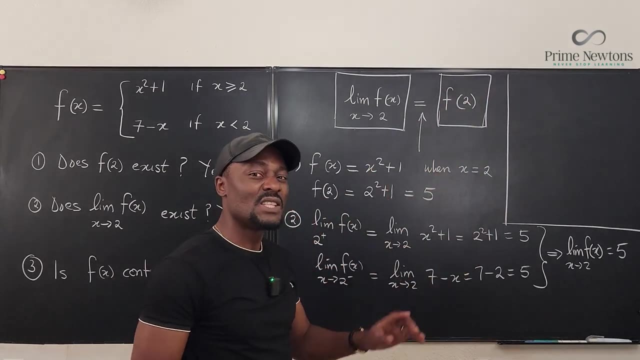 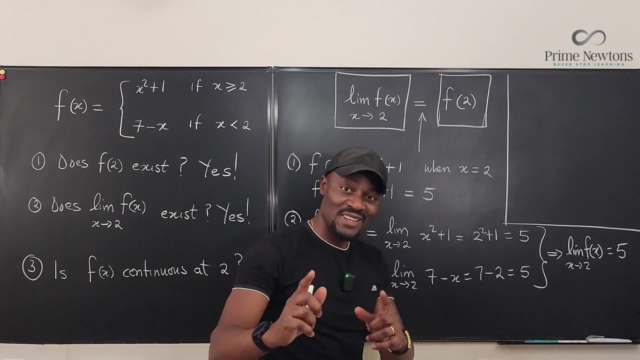 It's real. We can't change it. It's legit. So this is how you conclude: Because the limit of the function as x approaches 2 is equal to of the function at 2, it means the function is continuous at 2.. That's it, You're done. Go home and tell your parents you learned something, Okay, So don't.